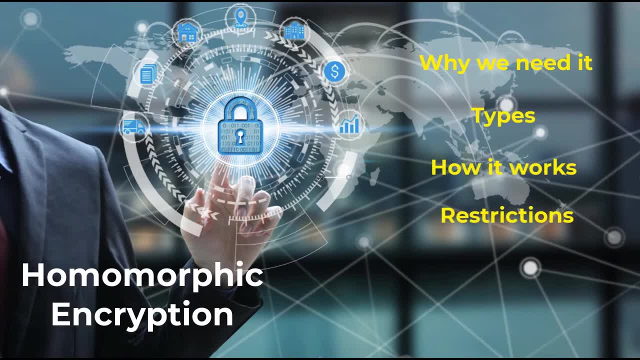 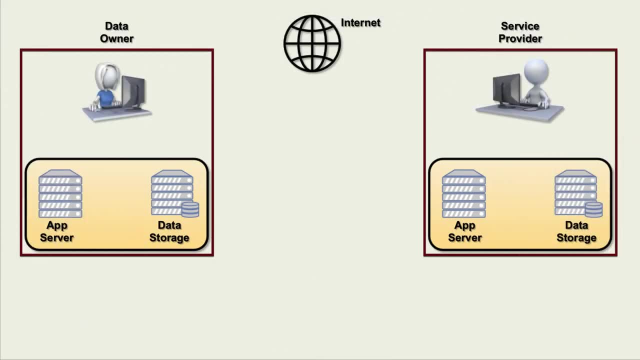 the types used, how it works and its restrictions. Encryption works with few issues when protecting data in transit and at rest. However, organizations today often share data sets with third-party processors- processors that provide statistical, marketing and other analysis requiring decryption of the data for off-premise use. 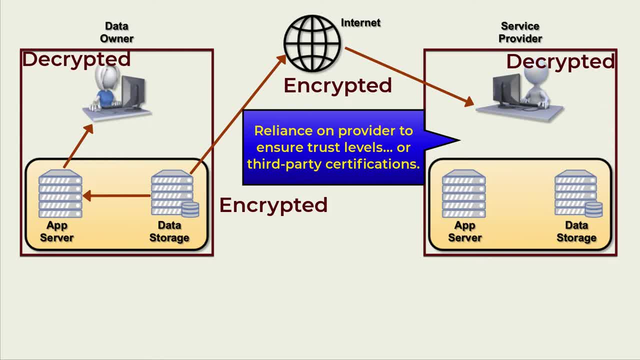 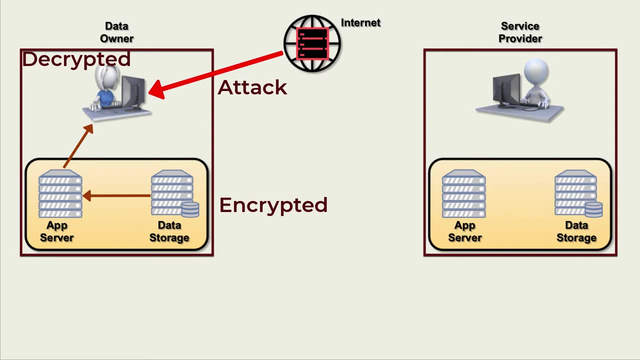 Making the raw and processed data available to threat actors over compromised media and systems. It isn't just off-site data we have to worry about. Data processed on-premise and over cloud resources is also decrypted, making it available to the inevitable intruder, As I explain later. 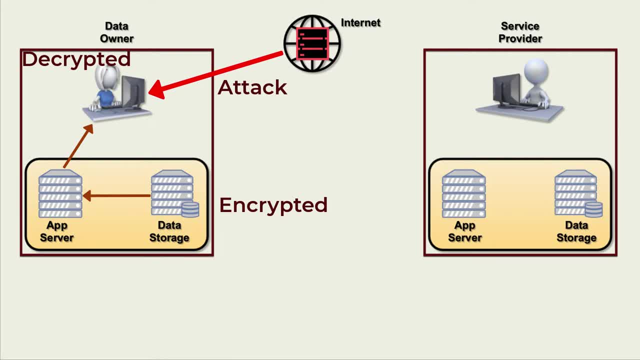 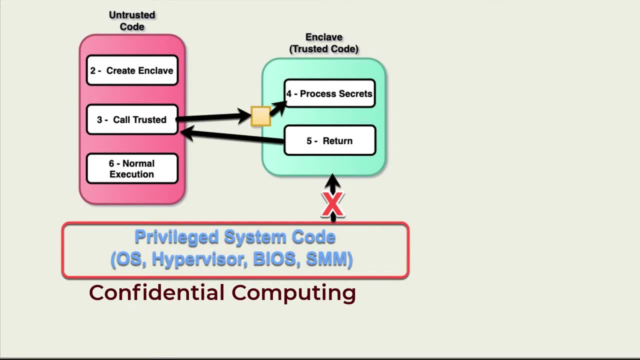 homomorphic encryption isn't ready for most applications yet, but it is moving in that direction. How to Protect Data. One solution to protecting data in use is confidential computing. Confidential computing, as shown here, creates protected spaces for processing decrypted data For a detailed. 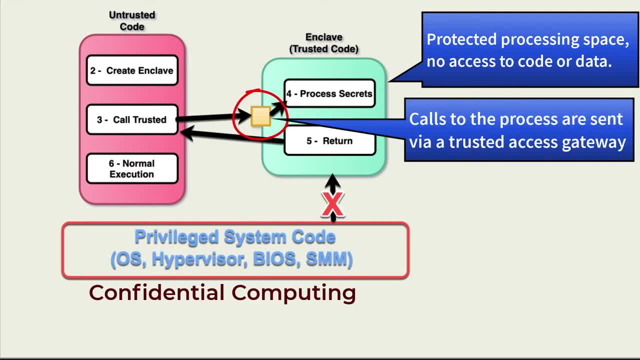 look at how this works. read the article at the link above. While this approach, being quickly implemented across organizations and cloud service providers, works well, it does not fully protect information that passes out of the control of the data owner, the organization that collects the data. 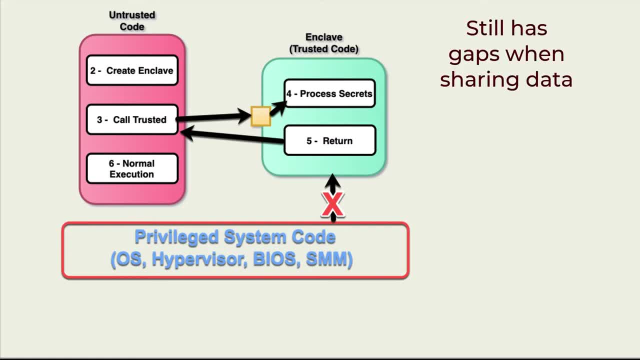 This makes compliance with privacy regulations like the GDPR difficult when data passes to potentially unknown storage locations- locations with trust levels outside the control of the data owner. Homomorphic encryption helps protect shared information by ensuring its encryption for the entire time it resides outside the data owner's control. There are three types of 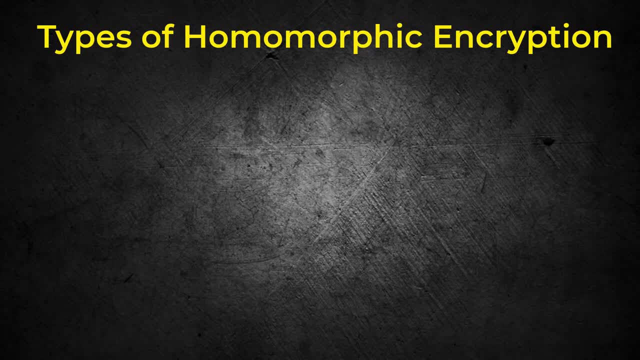 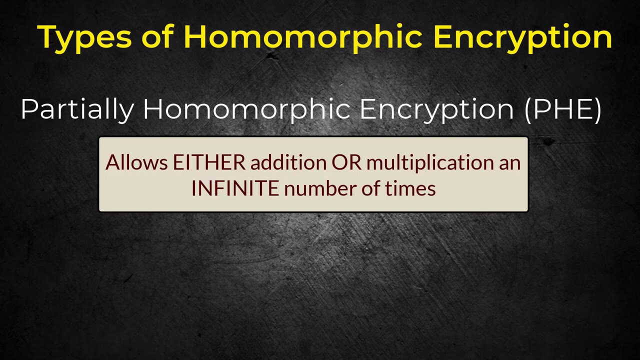 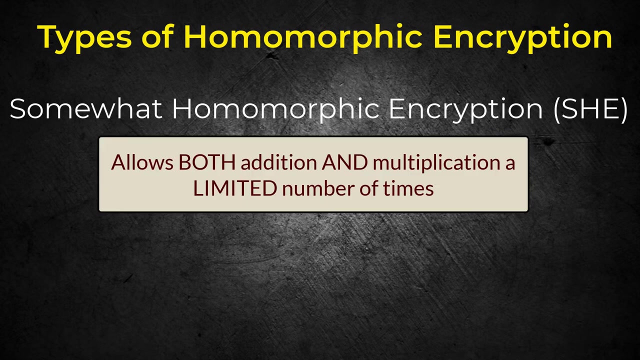 homomorphic encryption. The actions that can be performed on encrypted data depends on the type used. Partially homomorphic encryption, or PHE, allows either addition or multiplication an infinite number of times. Somewhat homomorphic encryption, or SHE, enables both addition and multiplication. 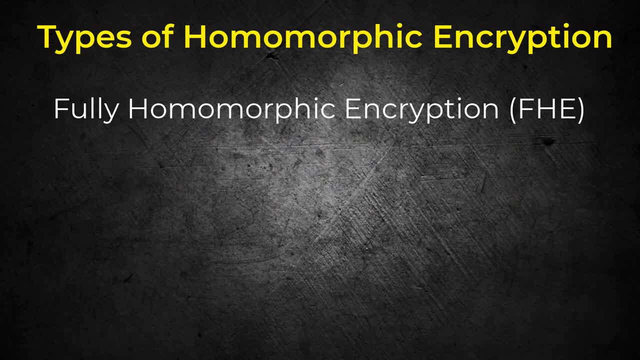 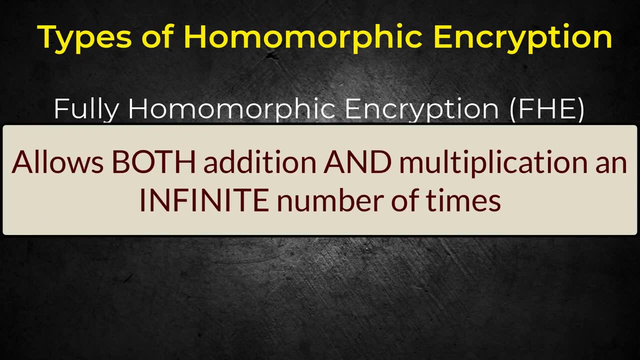 but restricts the number of operations performed. Fully homomorphic encryption, or PHE, can be used to protect data, but can't protect time and地ное. homomorphic encryption, or FHE, enables both addition and multiplication an infinite number of times. FHE is emerging as the type preferred by large service provider solutions like Microsoft. 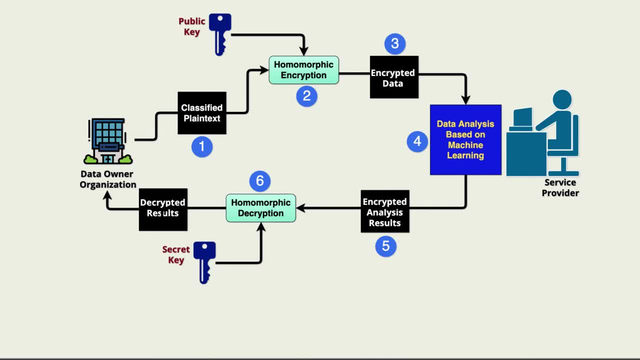 SEAL. In general, homomorphic encryption converts plain text into ciphertext, but it's ciphertext that can be accessed and processed without decrypting it. This approach requires the generation of not only keys for the data owner's encryption and decryption to plain text, but also 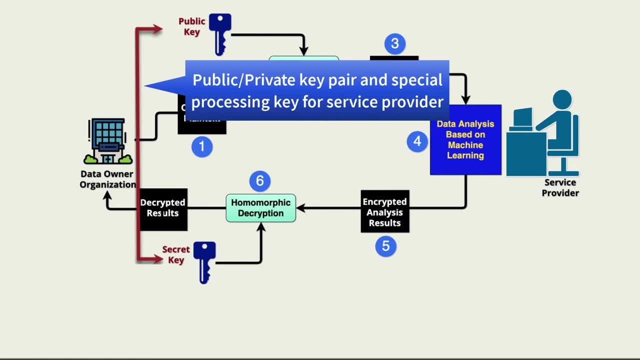 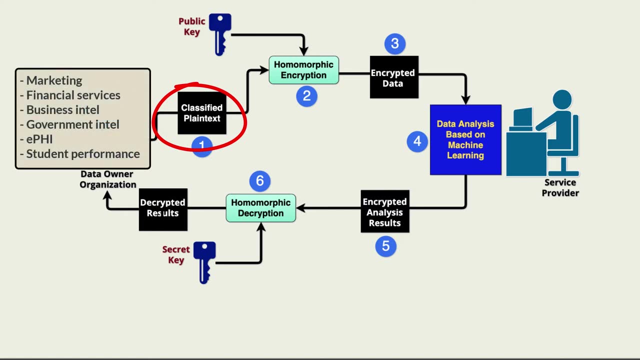 a key provided to the entity processing the information. Let's walk through how this works. The data owner creates a data set it wants to share for analysis. Examples include advertising and marketing, banking and financial services, business analysis and data analysis. The data owner creates a data set it wants to share for. 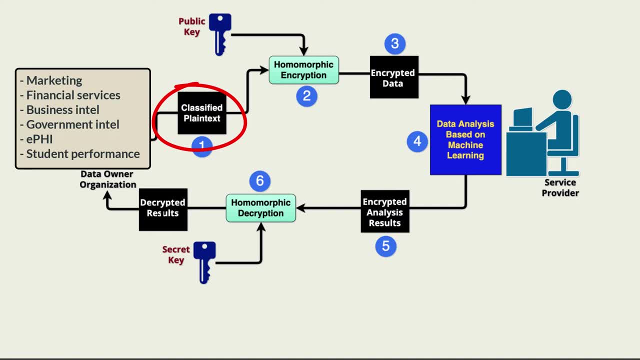 analysis. Examples include advertising and marketing, banking and financial services intelligence, government intelligence, electronic health care treatment records and student performance information. Second, the data owner designs a homomorphic encryption approach that enables access to the data elements that it wants analyzed. 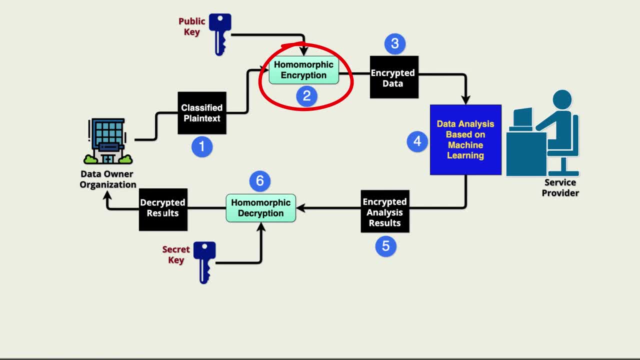 creating keys needed to encrypt the public key process, the homomorphic access key, and decrypt the data with the private key and the analysis. The design and key creation are usually done in collaboration with the service provider. The data owner then encrypts the data with the public key created for data sharing. 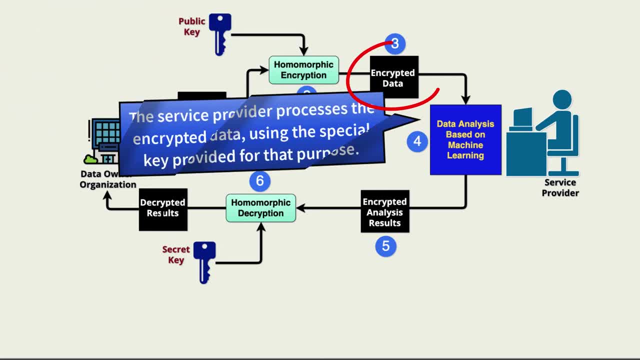 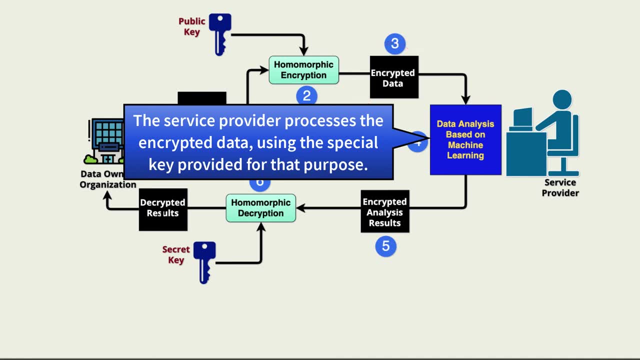 The homomorphically encrypted data is sent to the service provider along with the homomorphic access key. The service provider analyzes the data as agreed, but it is unable to see either the processed data or the results of the analysis. The still encrypted results are returned to the data owner and, finally, the data owner uses the. 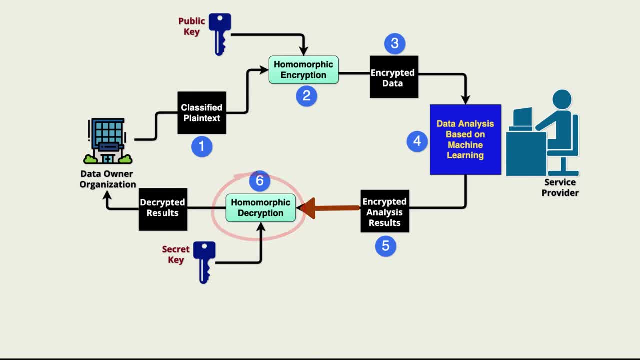 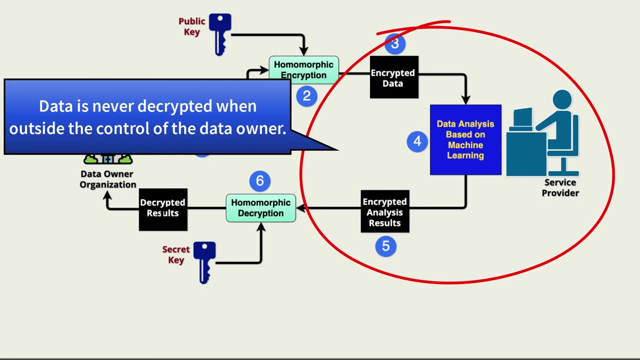 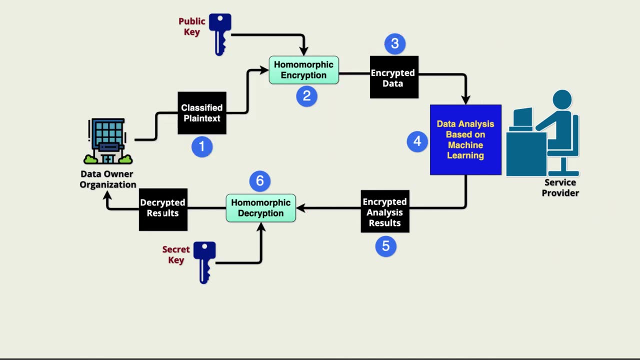 private key to decrypt the analysis. At no time is the data decrypted when outside the control of the data owner. This is a very brief look at homomorphic encryption. For a more detailed explanation, read my article at the link above. Homomorphic encryption is a resource hog. 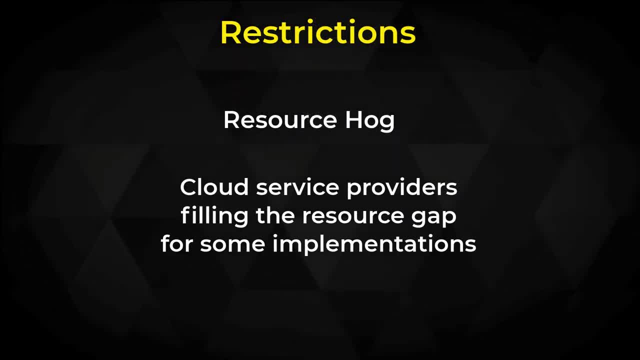 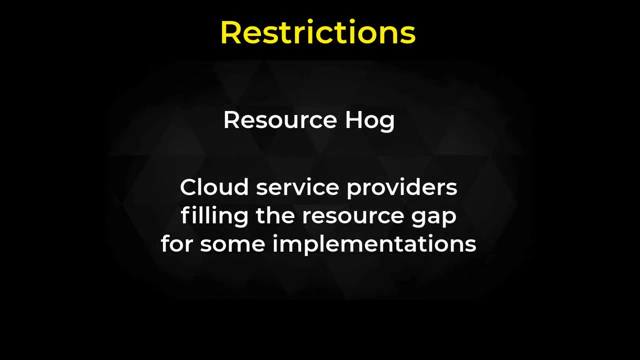 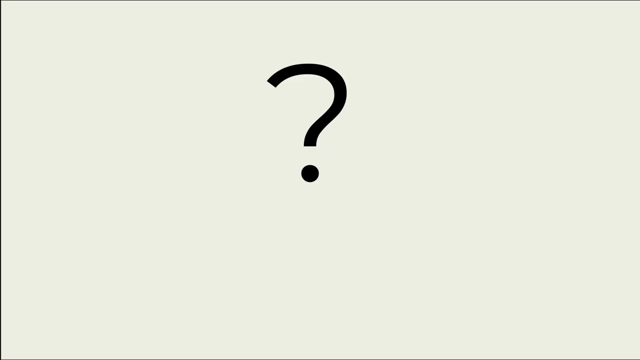 Making adoption for everyday processing out of the reach for the vast majority of organizations. This is why resource providers like those shown at the link above are emerging to enable its use across multiple industries and business sizes. Well, that's it for this lesson. If you have questions.